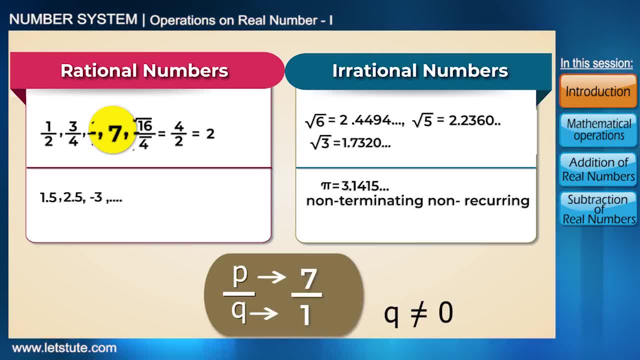 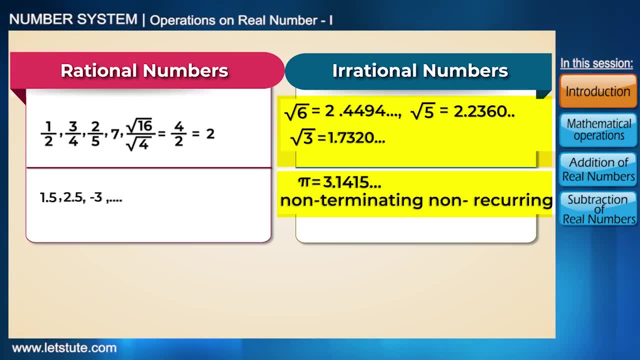 be written as 7 divided by 1, where p is equal to 7 and q is equal to 1.. Now, an irrational number is the opposite, one that cannot be written as a ratio of two integers. For example, root 6 is 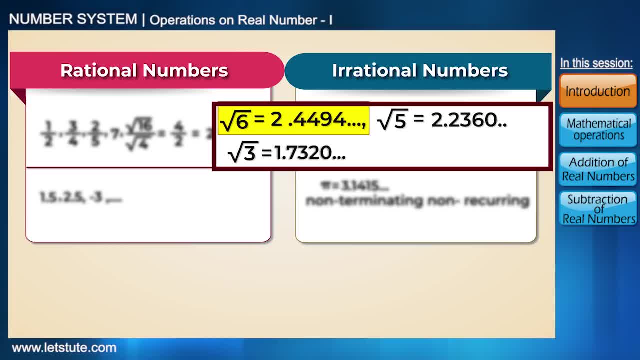 equal to 2.4494, and so on. Next, we have root 5 is equal to 2.2360, and so on. So all these are irrational numbers. All these are a non-terminating, non-recurring decimal. That is a decimal number. 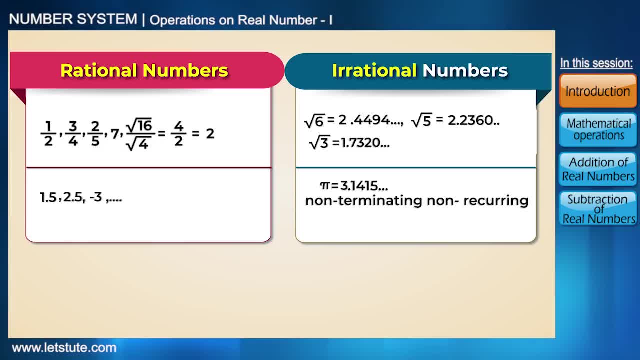 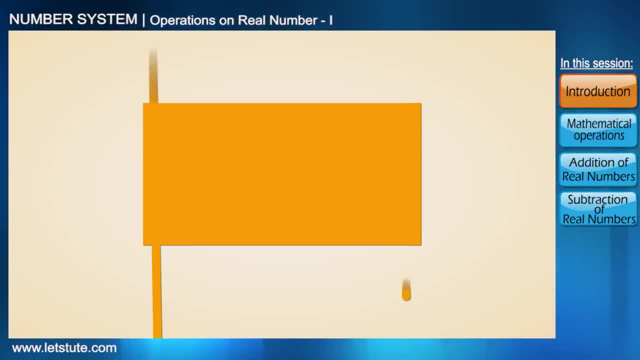 that never ends. The rational and irrational numbers together form the real numbers. In this session we are going to learn about the mathematical operation on these real numbers. Now we came to know what exactly real numbers are. But what are these mathematical operations? So the four basic mathematical 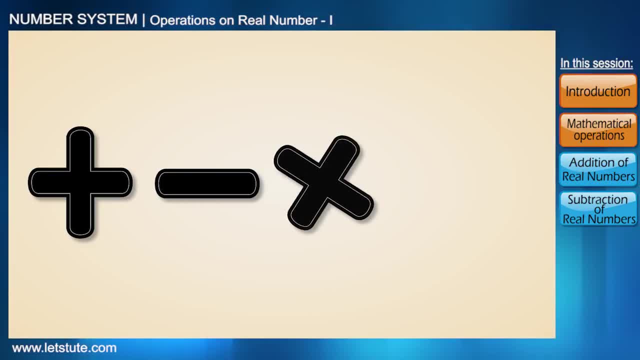 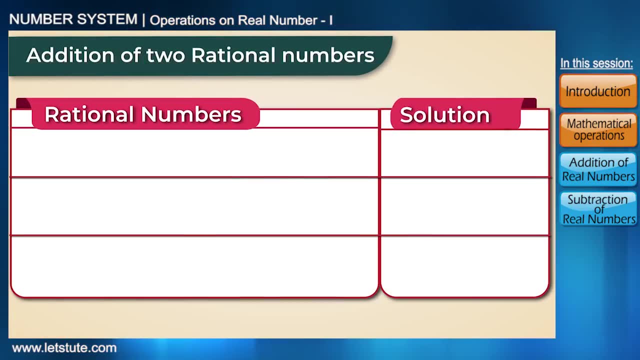 operations are addition, subtraction, multiplication and division. Let's see what happens if we add two rational numbers. Let's take an example: 0.24 plus 0.60, which equals to 0.84, which means we can write 0.84 in the form: 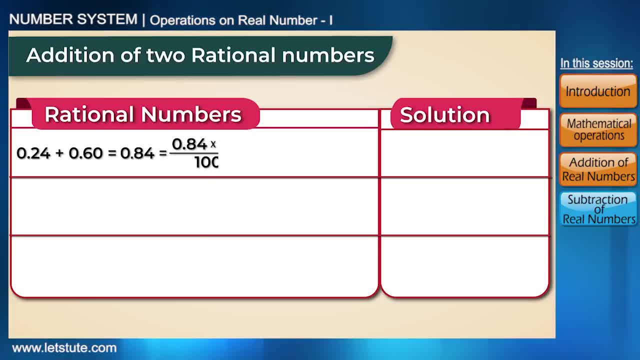 of p by q, that is 84 divided by 100, which gives solution as 21 divided by 25.. Here we are getting numerator and denominator as an integral, So we can write 0.84 in the form of p by q, that is 84. 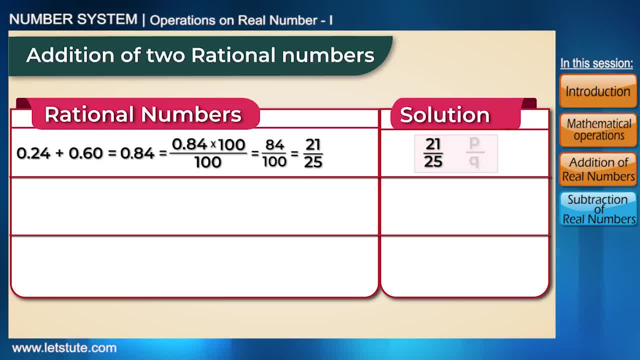 divided by 0.84, that is eight, so we get 0.84.. So we can write 0.84 of that equation and therefore 0.84 is the radical proof of theically number. Surely the following Countdown that: 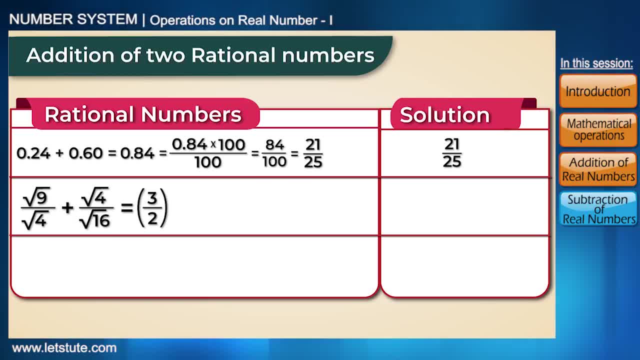 I've given here is the Ctrlri with King, n, Ln and Ne. So if there are two character inversion terms like hashes, gehen and muут- and they used to be the maximum interval wort Tekker use for this equation, Instead of that, the term q has been changed, That is, if, if the women change their position. as they change the position and raise the upper part. this term q is replaced by the tender position objects plus the bottom part, quef, so this term q is going to be less Tsaven. In this case, we now have two terms, and that is the 2021 and festival of five days in Thomas. 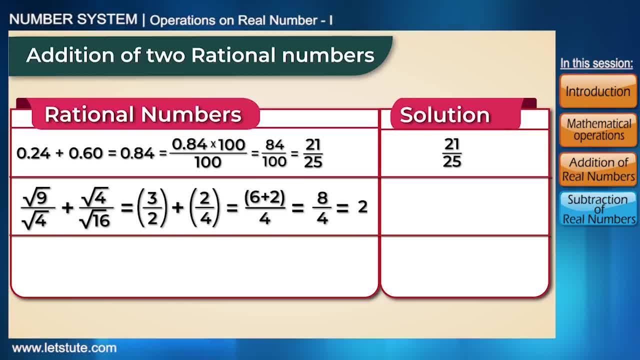 8 divided by 4, which equals to 2. so here again we can write it in the form of P divided by Q, that is 2 divided by 1. so 2 is equal to P and 1 is equal to Q. next example we are getting, again in the form of P by Q, that is 49 divided by 20. 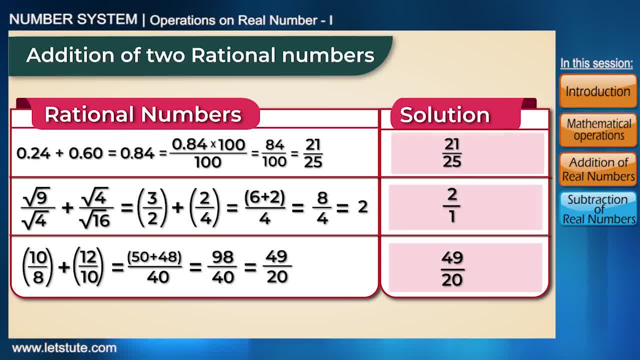 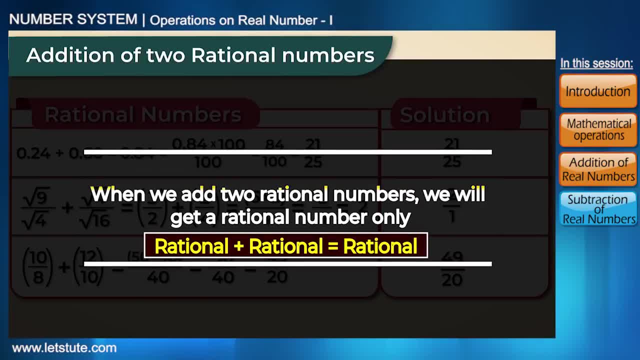 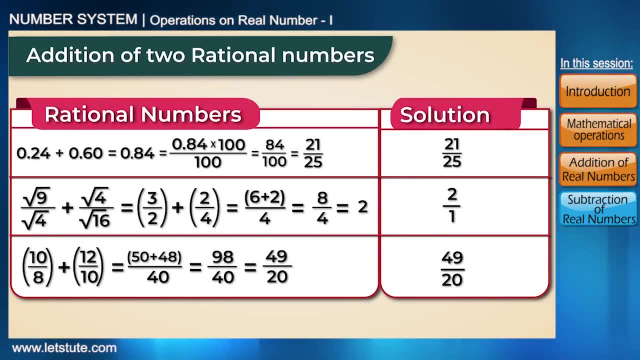 therefore these are all rational numbers, as we are getting the solution in the form of P by Q. now we can here say that when we add two rational numbers, we will get a rational number only. this is the first property of addition of rational numbers. let's move to the next case, when we have irrational numbers: root 3 plus. 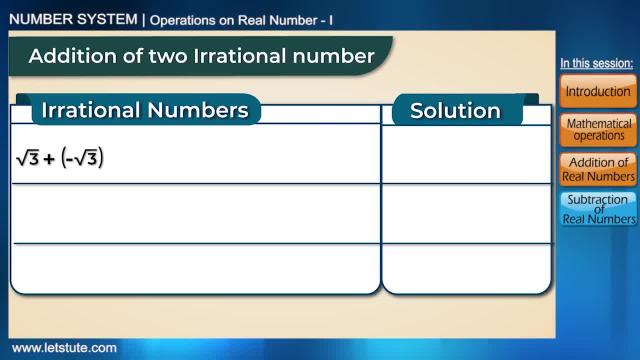 minus root 3, we get a solution equal to root 3 plus minus will be minus root 3, equal to 0. that is, we can write it it as 0 divided by 1, which is the form of p by q. hence it is a rational number. let's take another. 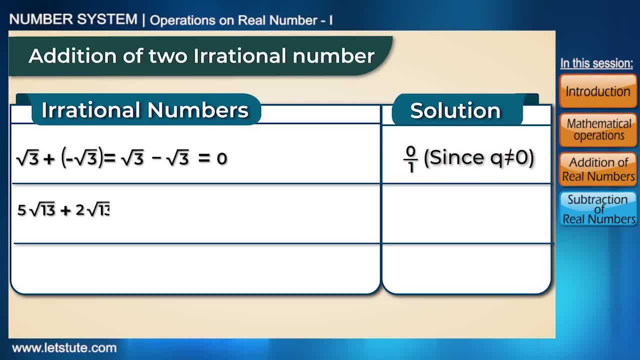 example: 5 root 13 plus 2 root 13, we get 7 root 13, equal to 7, into the value. of root 13 is 3.6055, and so on is equal to 25.2388, and so on. next example: so here, as we are getting non-terminating, 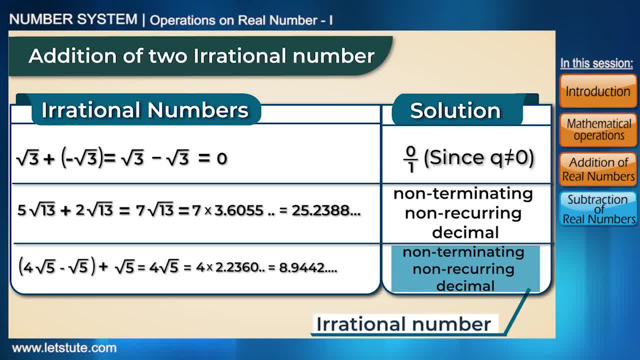 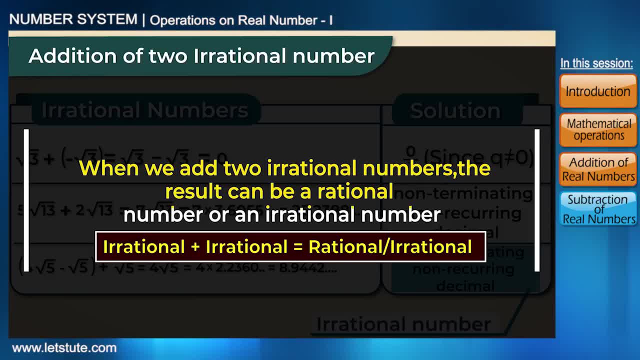 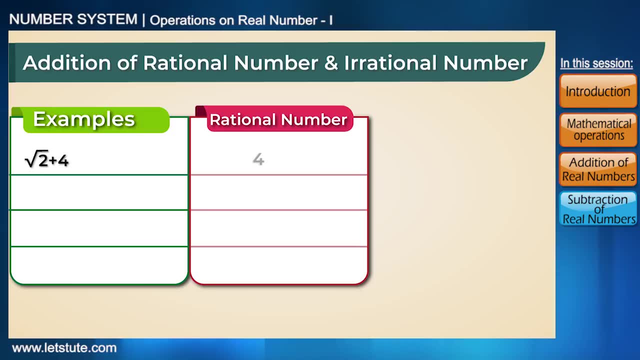 and non-recurring decimal, hence it is an irrational number. thus we can conclude that when we add two irrational numbers, the result can be a rational or an irrational number. now let's see what we get if we add rational number with an irrational number. so we get 25.2388, and so on, is equal to 25.2388, and so on is equal to 25.2388, and so on. 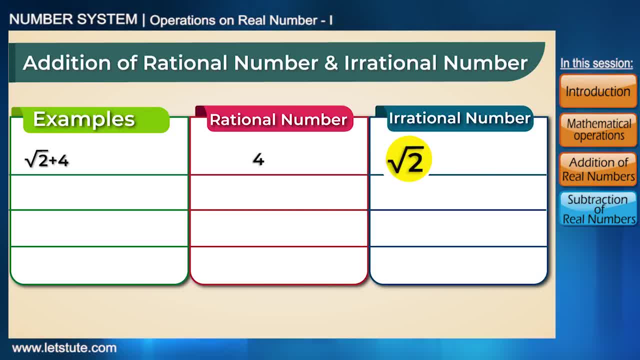 so here, when we add root 2, which is an irrational number, 4, which is a rational number, then we get: the value of root 2 is equal to 1.4142, and so on plus 4, this will give us 5.4142, and so on. 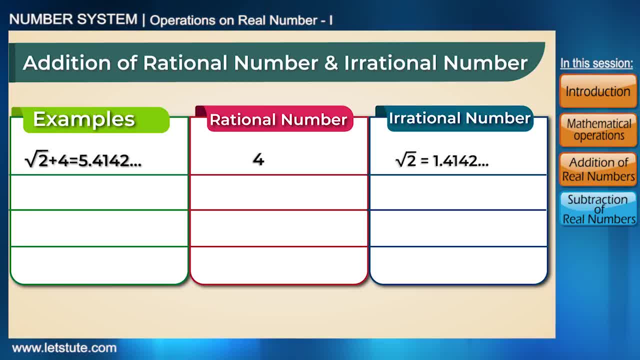 that is a non-terminating and non-recurring decimal, which is an irrational number. similarly, let's take another example: root 13, which is an irrational number, plus root 4, which is a rational number, we get the value of root 13 is equal to 3.6055, and so on plus. 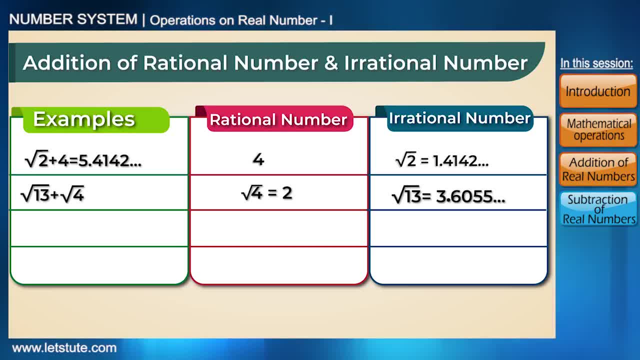 root 4 is 2, which will give us 5.6055 and so on. that is again a non-terminating and non-recurring decimal, which is an irrational number. similarly, we can see in other examples: we are getting solution as an irrational numbers, hence the additional number, which is an irrational number. 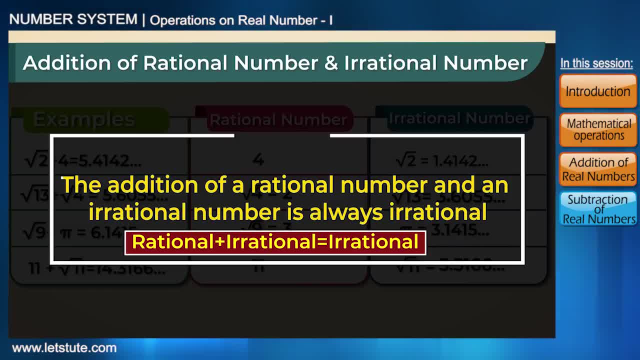 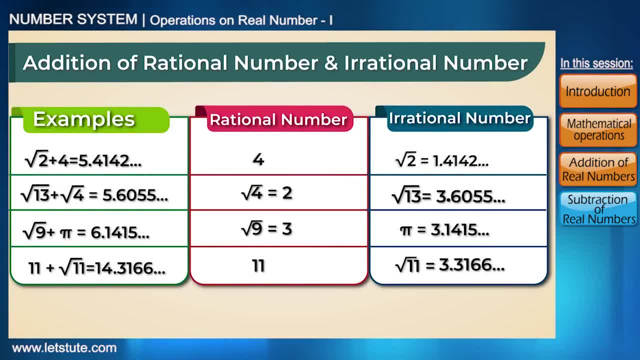 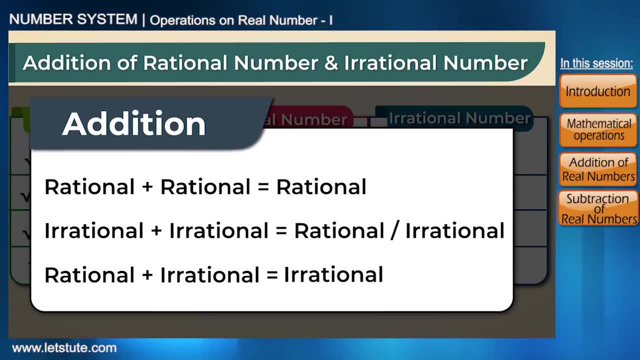 plus the addition of a rational number, and an irrational number is always irrational. so this is our third property of rational numbers. okay, friends, this was for addition of real numbers. the same results are obtained when we do the subtraction of real numbers. why don't you guys try few of these subtractions of real numbers and let us know the answers? 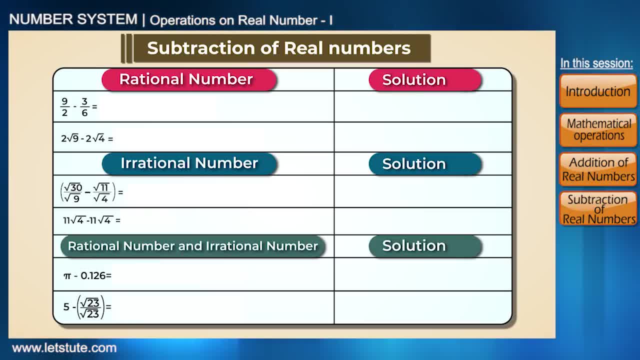 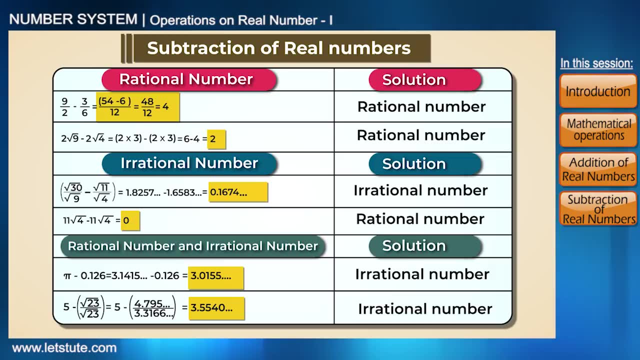 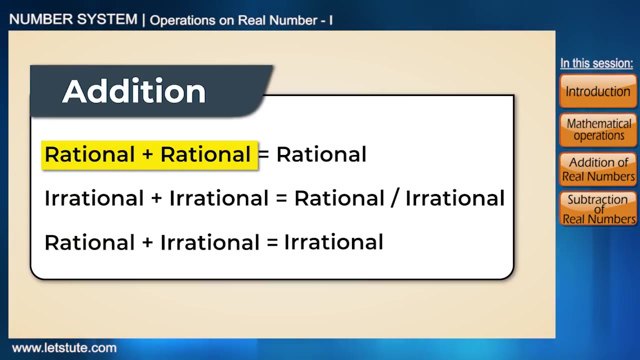 and also let us know that: does these properties really hold true for subtraction too? well, you can see here: this property hold true for subtraction too. so what we have learned in this session: if we add two rational numbers, then we will get a rational number only. next. 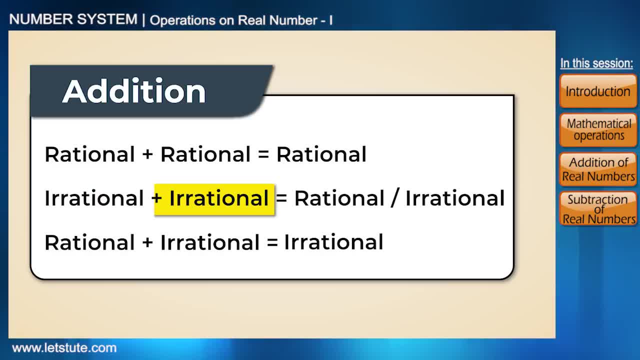 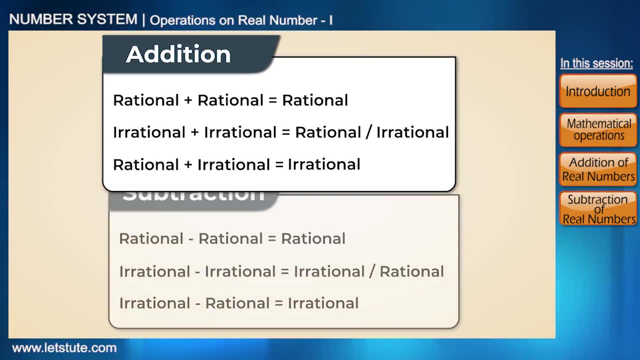 if we add two irrational numbers, then the result can be a rational or an irrational number. and at last we have seen: if we add a rational number and irrational number, then we will get a irrational number. and this property hold true for subtraction too. so, friends, in the next session we are going to learn about remaining properties and also 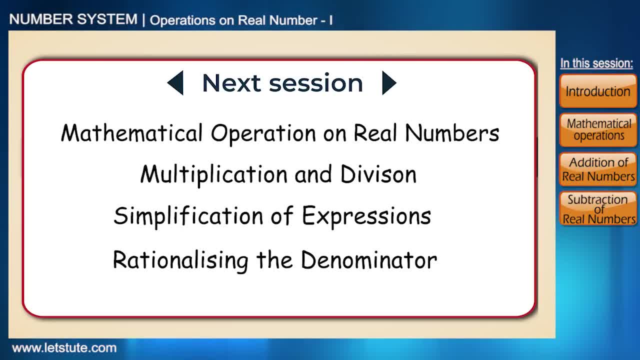 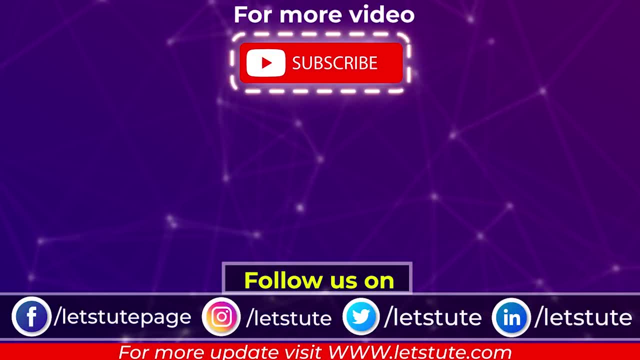 we are going to see how to simplify the expressions and how to rationalize the denominator. i hope you guys have enjoyed the session. don't forget to hit the like button and comment down if you have any queries, and we will see you guys in the next session. bye, bye.